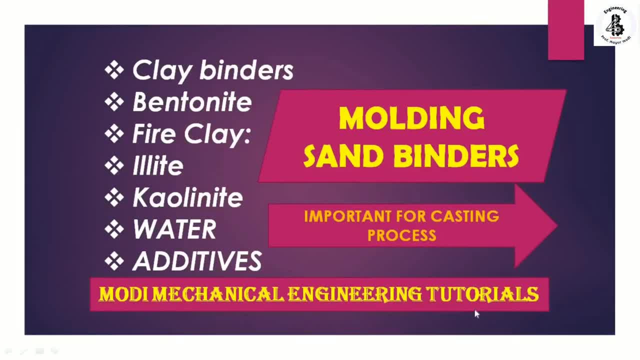 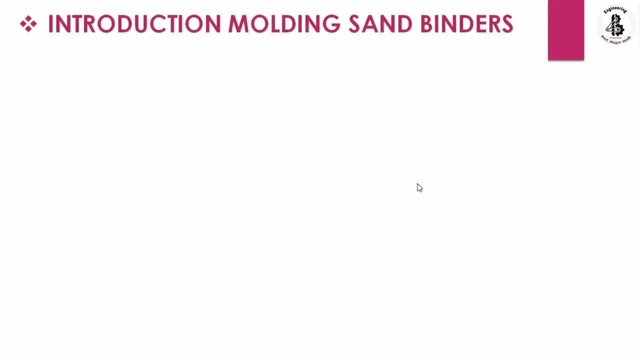 Welcome to my YouTube channel, Modi Mechanical Engineering Tutorials. In this video I would like to explain on Molding Sand Binders. So this is an important topic for casting process. So let us start with the introduction on Molding Sand Binders. So basically, binders produce cohesion between the molding sand grains in the green or dry state, or you can say that will be the two conditions of the sand. It will be indication as a green condition and dry conditions. So basically, binders gives strength to the molding sand so that it can retain its shapes as a mold cavity. 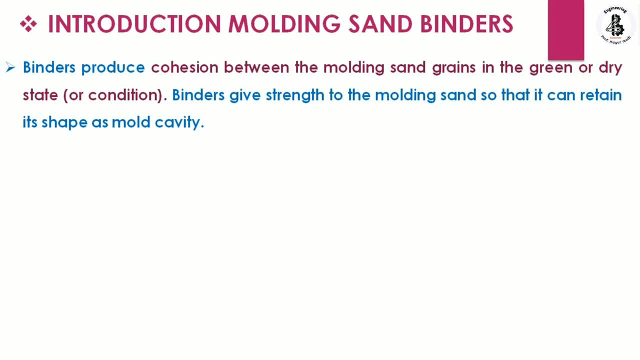 So, basically, this binder that will be used into the sand molding process, So that will be increasing the dimensional accuracy as well, as it will be not damaging the mold cavity, Or you can say it will be retain its shape as a mold cavity. So that will be the necessary conditions for sand molding process. 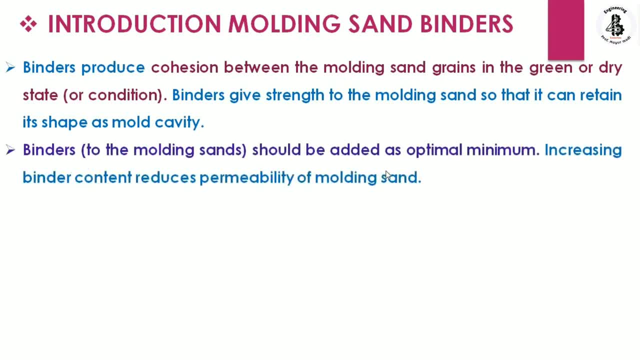 So binders should be added as optimum minimum. That's why that will be increasing the binder contents, reducing the permeability of molding sand, So as per the requirements of the binder, So such kind of concentrations is being added into a molding sand Then, and then it will be having a better accuracy. 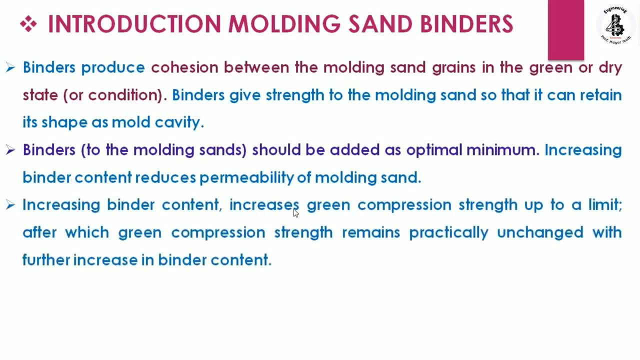 Increasing binder contents increases green compression strength up to a limit after which green compression strength remains practically unchanged with further increasing binder contents. So, as per the my requirements, So such kind of concentrations of the binder, such kind of amount is being added, Not less than that or not more than that. 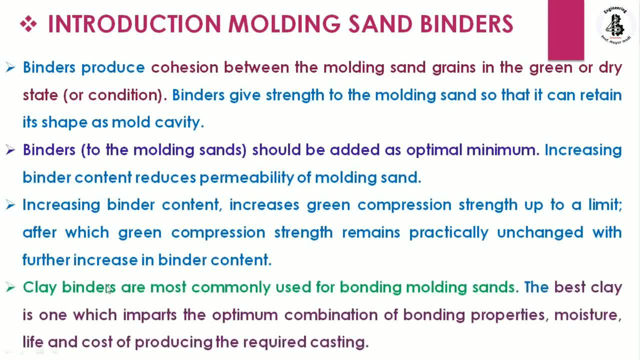 That will be the important part as a binder materials. So the clay binders are most commonly used for bonding the molding sands. The best clay is one which imparts the optimum combinations of the bonding properties, moisture, life and cost of the producing the required castings. 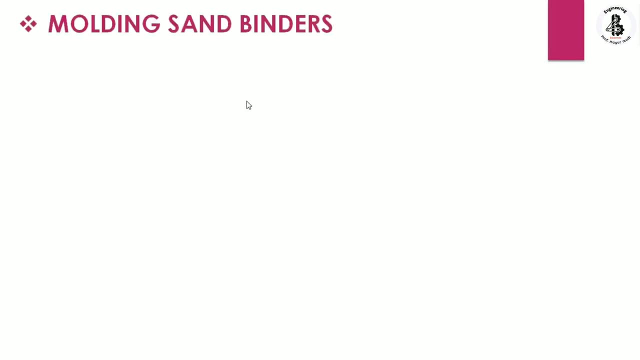 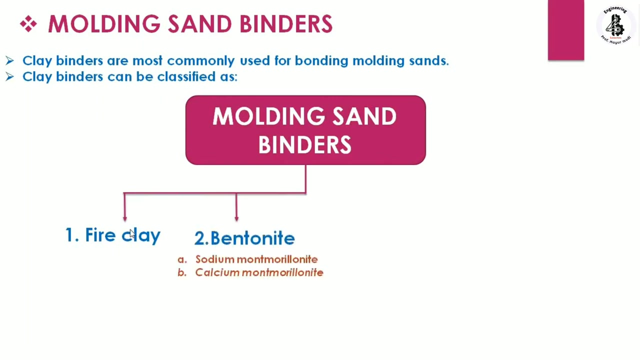 then molding sand binders. so basically, the clay binders are most commonly used as a bonding molding sense. clay binders can be classified as: so the molding sand binders. so first of all that will be a fire clay, second one bentonite. so basically, in case of the bentonite, 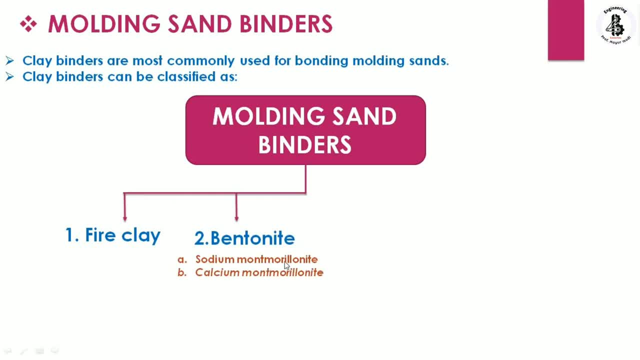 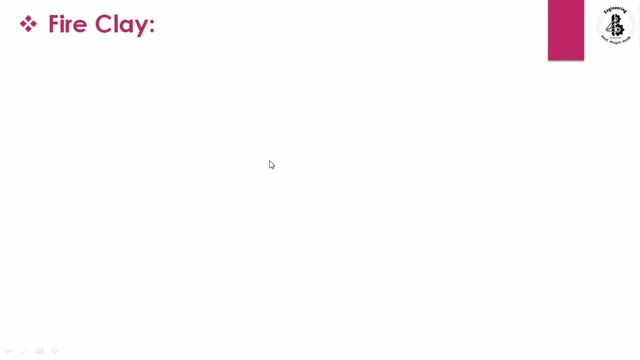 there will be the sodium montorilonite and calcium's montomerolinite, third one, elite, and last one as a molding sand binder, that will be kaolinite. so let us start with the each and every molding sand binders, so starting with fire clay. so basically, fire clay is a refractory. 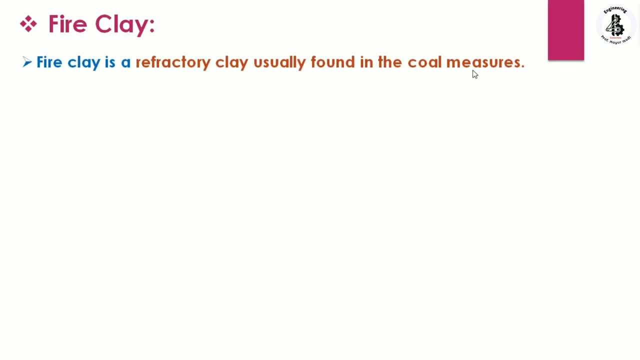 clay, so so. so found into the coal measures. fire clay particles are about 400 times as large as compared to those of the bentonite, so hence the same percentage of the fire clay produces lower strength. second one, bentonite. so in case of the bentonite is: 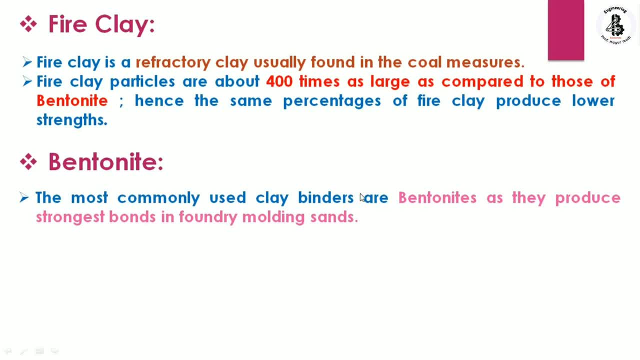 most commonly used clay binders and they produces strongest bond in the foundry of the molding sand. so that will be having the wide applications in the field of the casting process. bentonite deposits are available in India, basically into Rajasthan and Bihar. bentonites are the weathered products of volcanic ash. 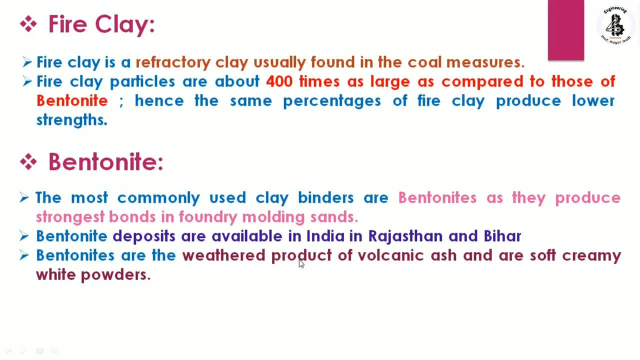 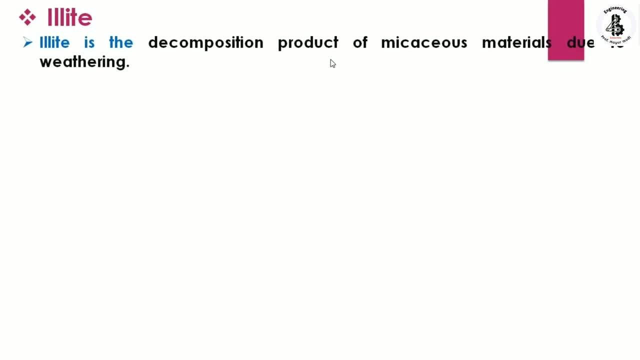 and are soft creamy white powders. then third one, alight. alight is a decompositions products of mucous. materials used due to the withering alight is found in natural molding sands. light has softening point around 2500 degree Fahrenheit. light does not swell in the 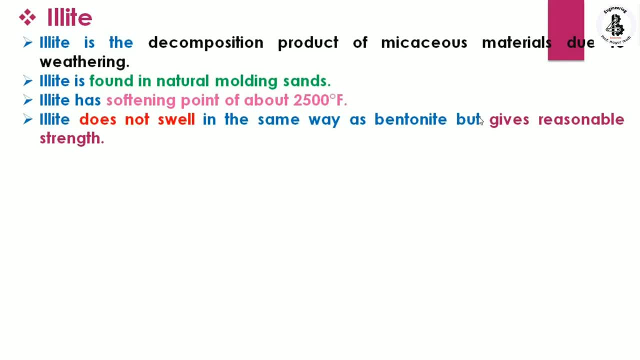 same way as bentonite, but it gives the reasonable strength. alight particles have thickness and width of 20 and 100 to 250 milli microns respectively, kaolinite. so basically, kaolinite is the residue of the weathered granite and basalt. 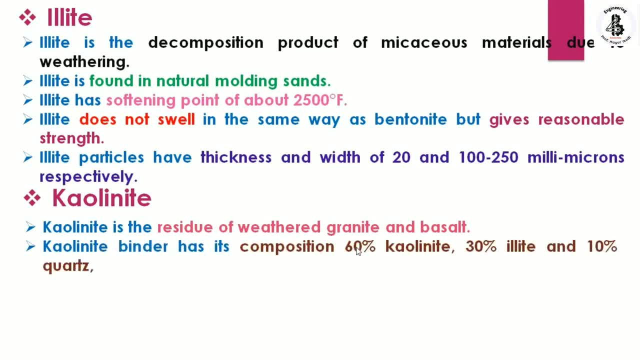 bentonite binders had its compositions around 60 percentage of kaolinite, 30% of alight and 10% of the quartz. kaolinites gets very slow swelling due to the water and is non gel forming. so that is the characteristics: kaolinites particles. 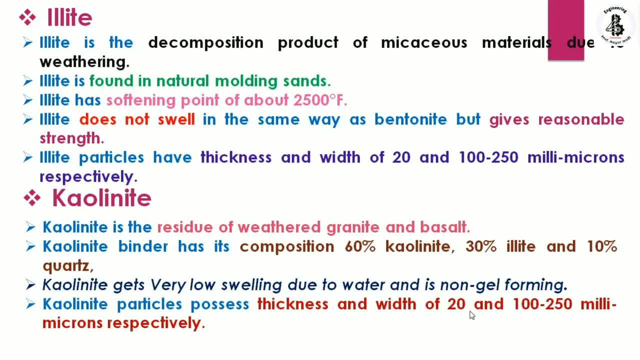 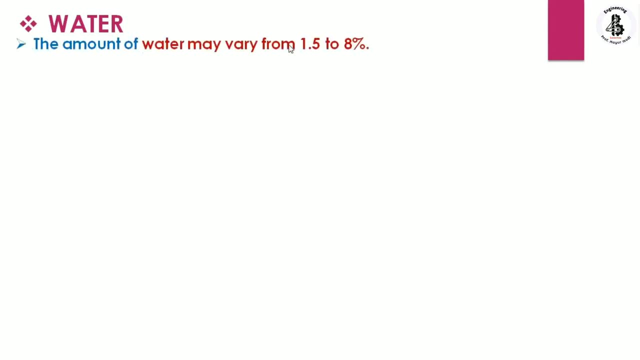 processes thickness and a width of 20 and 100 to 250 milli microns respectively. so it will be similar to the alight characteristics. then the amount of the water may be very, from 1.5 to 8 percent. so that will be. It depends upon the 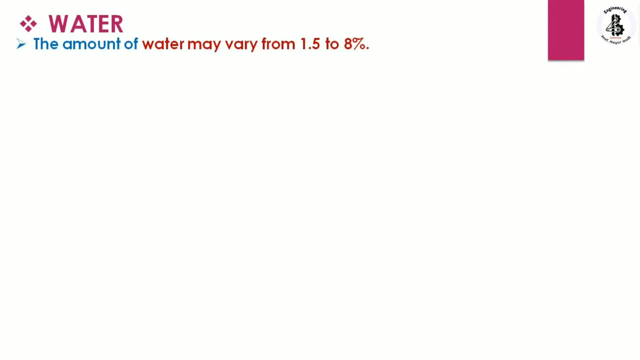 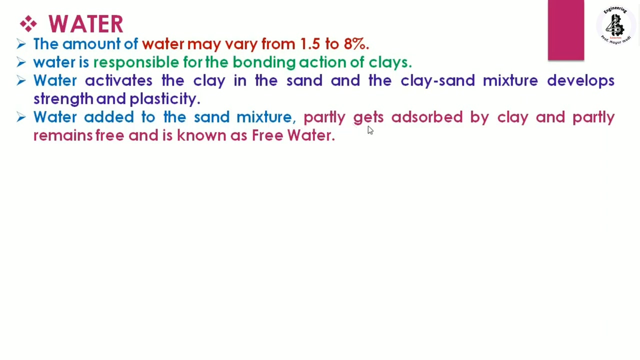 conditions of the sand, It will be green or dry. Water is responsible for bonding actions of the clay and water activates the clay in the sand and the clay sand mixture develops a strength and plasticity. So due to that, water added to the same sand mixture partly gets absorbed by the clay. 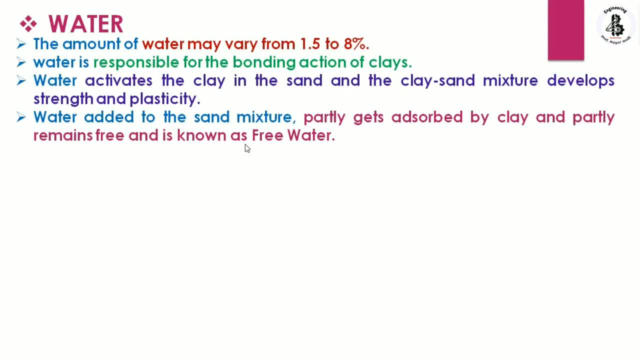 and partly remains free and is known as a free water. The absorbed water is responsible for developing the proper bonds and green strength. The free water acts as a lubricant. so by the these free waters, these sands, it would be easily filled around a pattern for making a sand mold, So it increases plasticity. 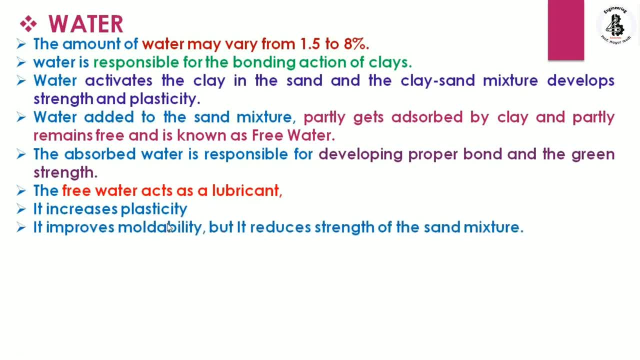 it improves the moldability, so that would be easily converting the sand molds, but it reducing strength of the sand mixes. so due to that free water for a given type of clay and its amounts, there is an optimum required water content. so as from the requirements of that particularly, 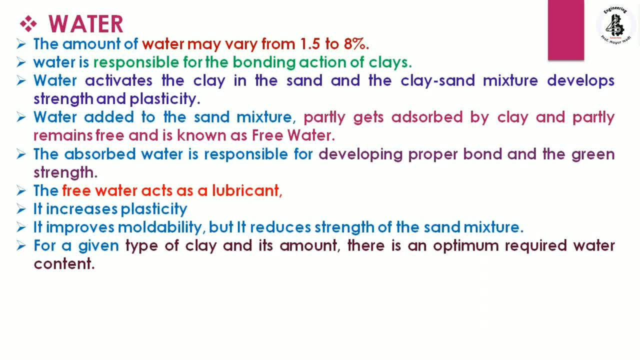 plasticity and lubrications onto that sand. the such kind of compositions or percentage of the water- maximum up to the eight percentage it will be added into the for making a sand mold. too little water will not be developed the proper strength and plasticity if it will be the less. 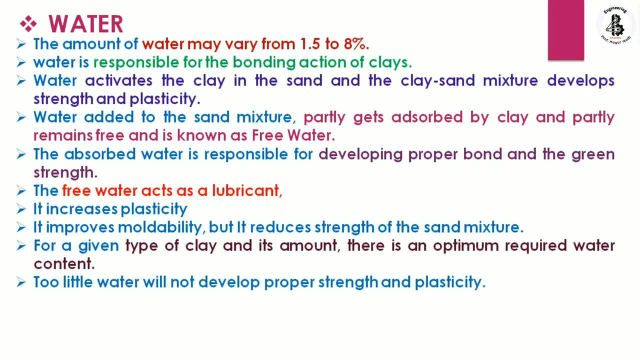 amount of water is being added, so that will be having a low flow characteristics, low strength and low plasticity, so that will be difficulties for making a mold cavity. too much water will result in excessive plasticity and dry sand. the amount of water required to develop the optimum properties. 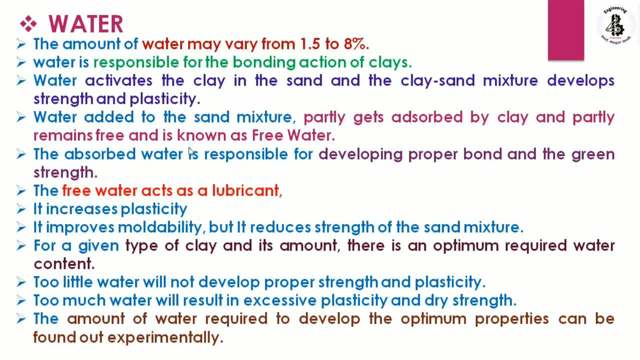 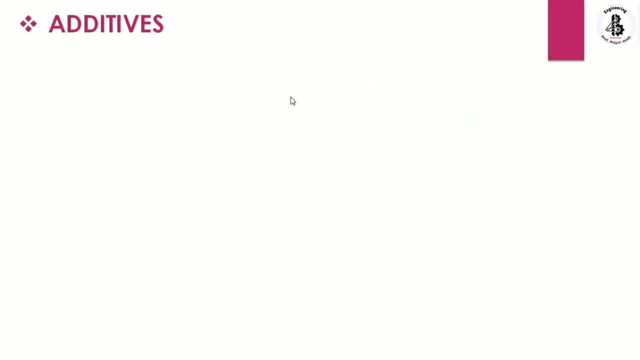 can be found out experimentally. so as from the requirements, it will be added maximum up to the eight percentage. then additives: the basic constituents of the molding sand mixtures are sand binders and water. so by the application of these three it will be the sand making process, the materials other than the basic ingredients. 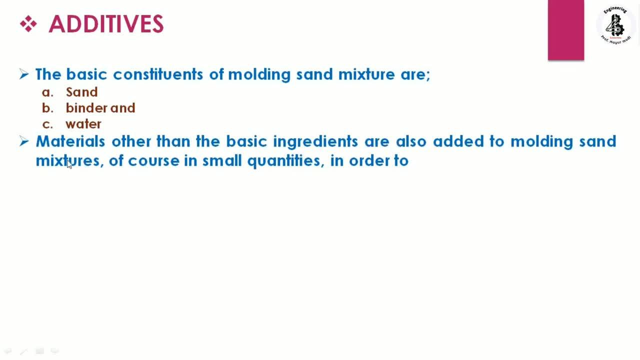 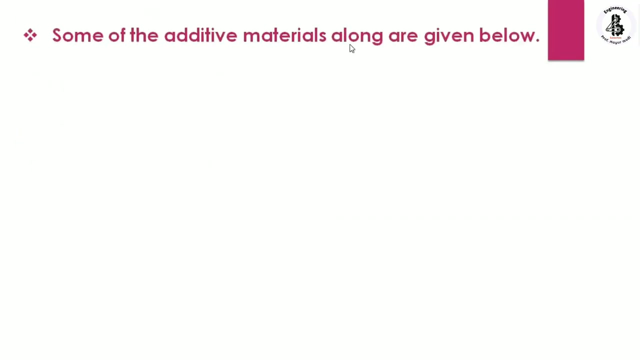 are also added to the molding sands mixtures, of course into the small quantities, in order to enhance the existing properties, to develop the certain other properties, to give the special qualities like resistance to sand, expansions, defects, etc. some of the additives of the materials alongs are given below the facing materials. 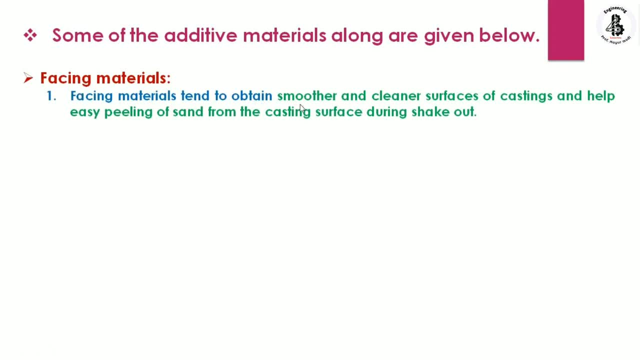 so, in case of the facing materials, tends to obtain the smoother and cleaner surfaces of the castings and help easily peeling of the sand from the casting surface during the shake out. second one: a few facing materials are sea coal, graphite, coke, silica floor, then cuisin materials. so, in case of the cuisin materials, burns when the molten metal is poured.